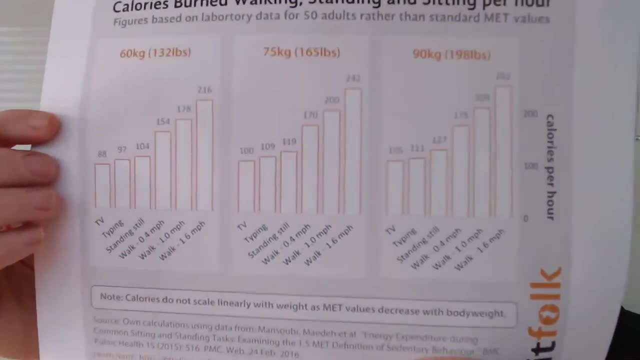 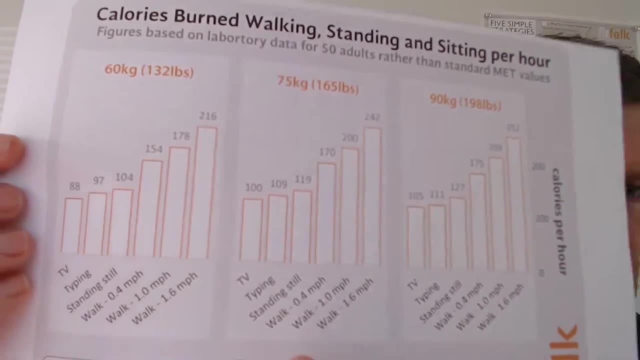 someone standing still and someone walking at different speeds. So you'll see that this I've kind of compared it across three different weight ranges, but we're just going to go with the one in the middle. Focus on that and you'll see that kind of here. this is watching TV. this is typing. 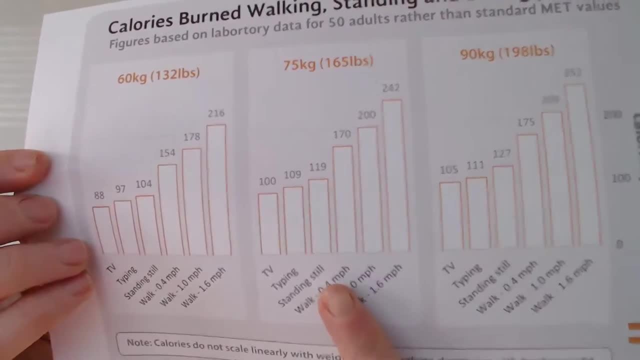 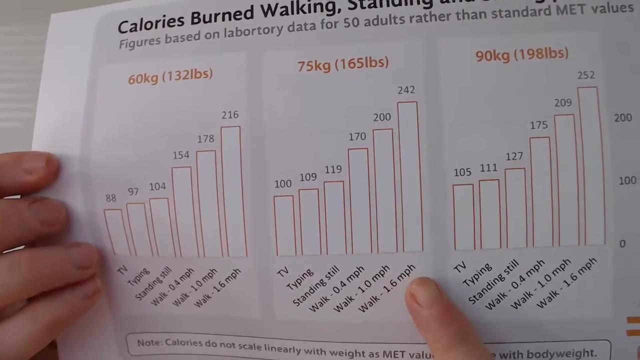 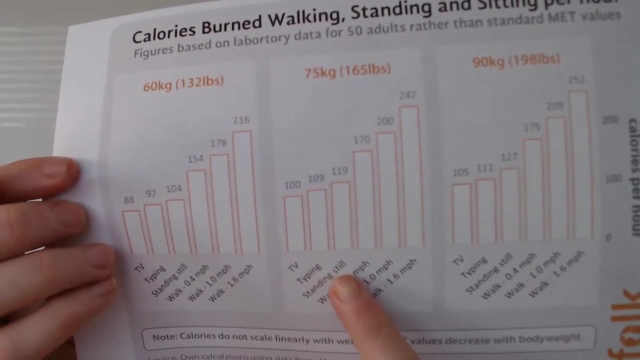 this is standing and then you've got walking at three different speeds. So walking slowly, walking a bit more quickly and walking, and basically you can see very quickly, as you stand up and start walking, that your calorie burn increases. But for standing up, going from sitting to standing up, it's a pretty minimal increase and 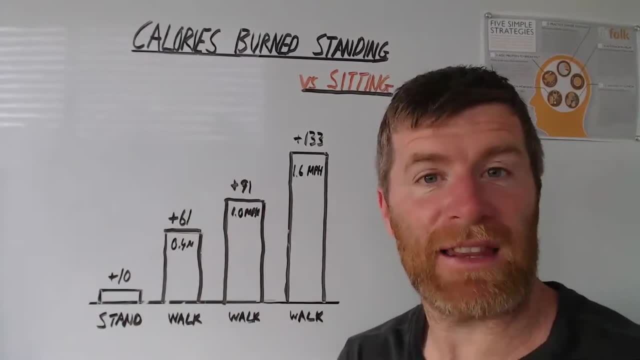 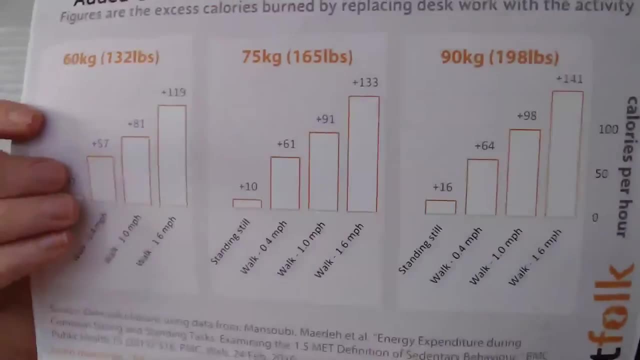 to make it more obvious. what I've done here is I've netted out the values, So I've taken away the energy that you burn while you're sitting, and this will give us a comparison of what we get kind of from standing walking, walking more quickly and walking fast, And you can see that. 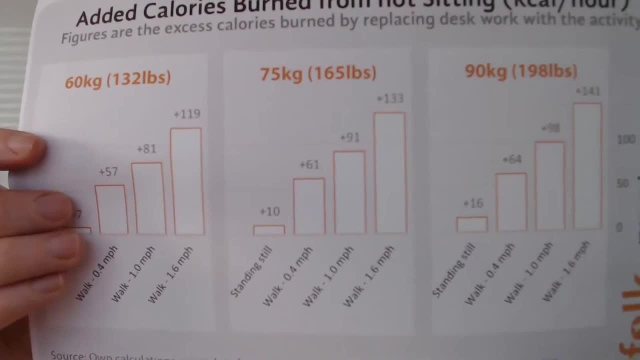 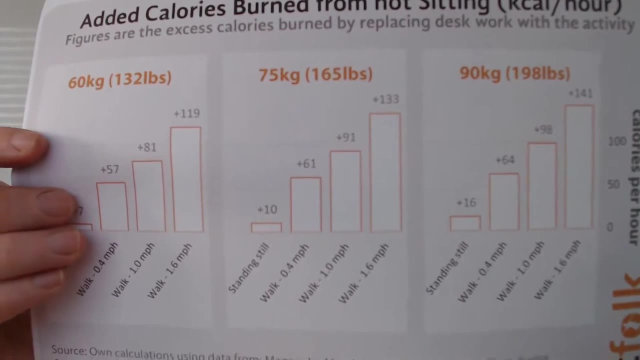 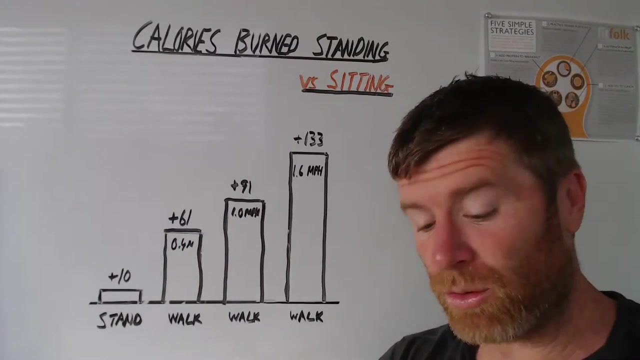 you're only adding kind of 10 calories per hour. really, It's really nothing. So it's a very, very minimal additional calories. So that's calories burned per hour and this is what I've shown here. So basically, when you go from sitting to standing, so the argument for a standing desk: 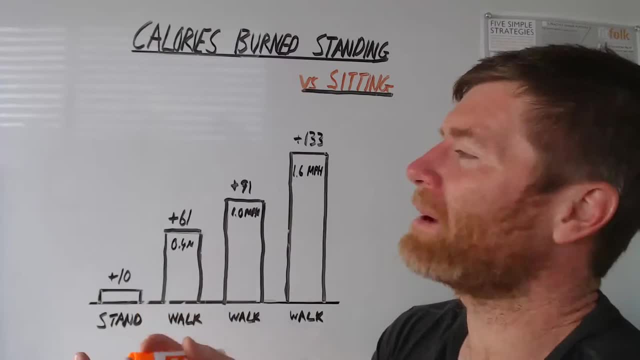 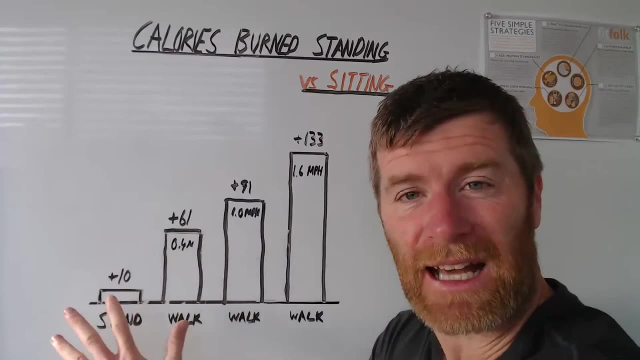 that you might burn more calories is very, very limited because basically, once you stand up, you're still just bearing all the weight On your joints and your body is remarkably efficient. You're only adding 10 calories per hour Now, 10 calories per hour in the context of a normal person that burns two to three thousand. 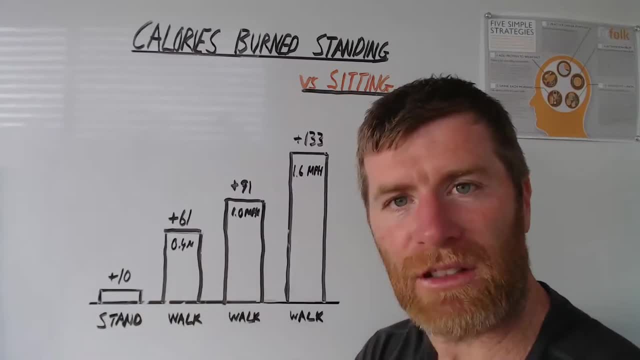 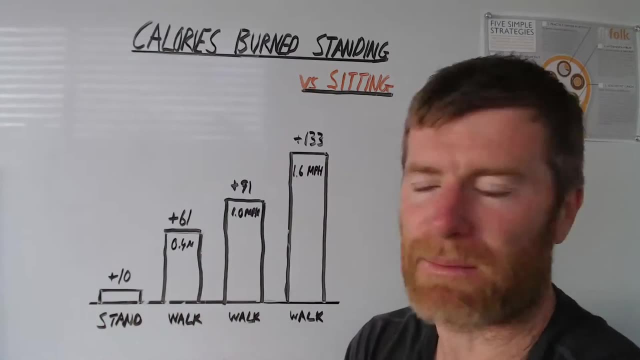 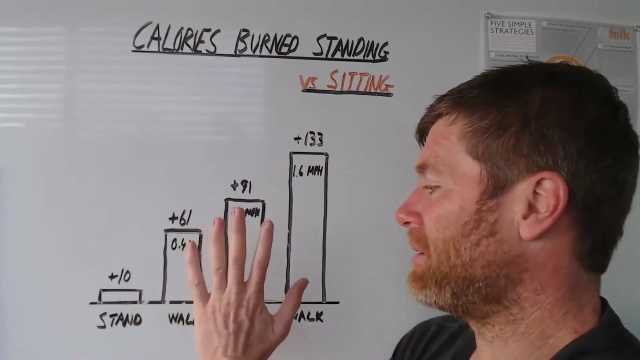 calories is nothing. So in terms of calorie burn, the argument for a standing desk is pretty minimal. in terms of, you know, posture or health, perhaps is a better argument Once you start walking. so the argument for a treadmill desk is much, much more solid. So once you start walking slowly, 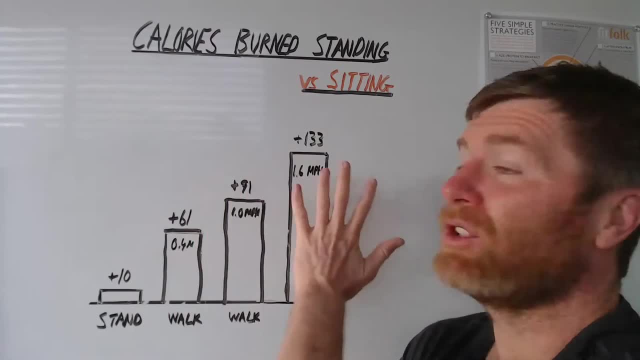 it's an extra 60 calories, Now, more quickly, another 90.. And then, if you're walking quickly, there's 130 calories an hour. So this is why you, you walk, you add your knee. This is actually really and it's phenomenally. 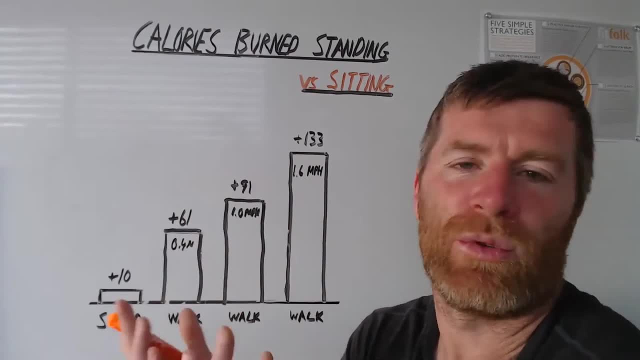 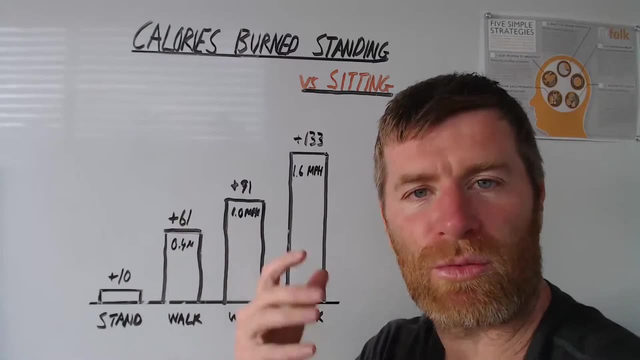 healthy. So the argument for a treadmill desk: I personally wouldn't work at a treadmill desk because you know it's just not very productive for me. But if you can make phone calls while you walk, if you can do walking meetings, if you can walk work at a treadmill desk, then that's quite. 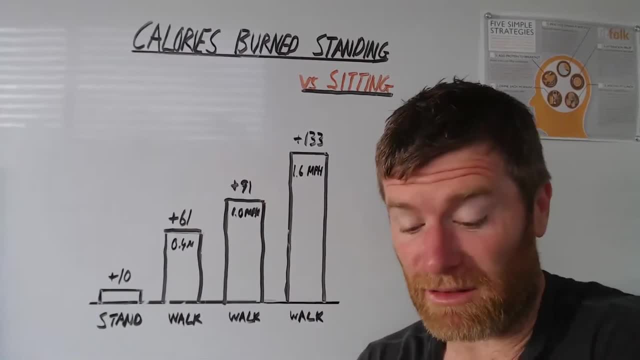 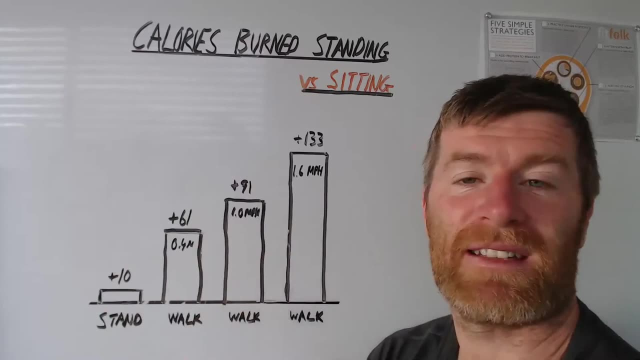 useful, But a standing desk not so much. It's really not a calorie burner, And that is what the data tells us. So if you're walking, you're not burning calories. So if you're walking, you're not burning calories. So it's very simple. But the calories burned standing as opposed to sitting. 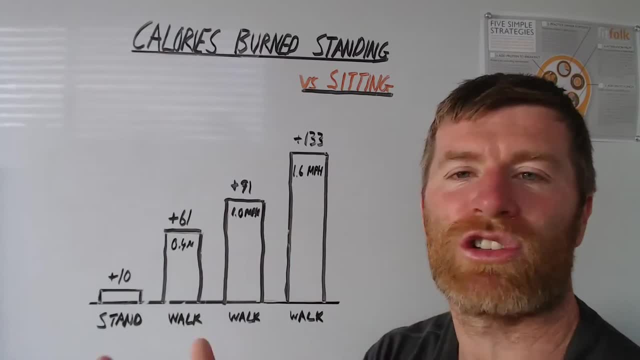 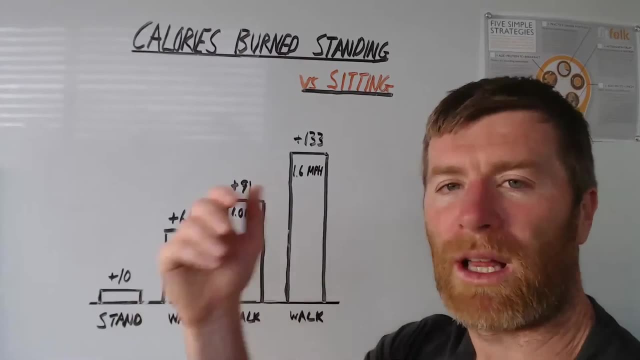 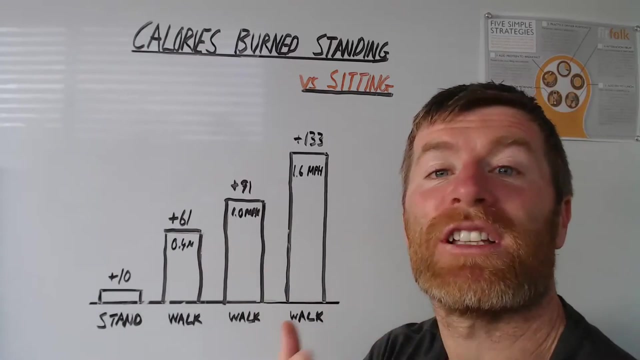 a very, very minimal extra 10 calories an hour, So it shouldn't really factor into your calculations about whether you stand or sit for your work. You're going to get more bang for your buck once you start moving because you are pushing the earth away. Basically it's gravity, So you can. 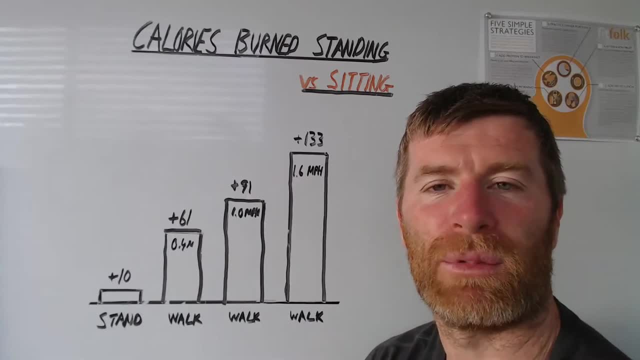 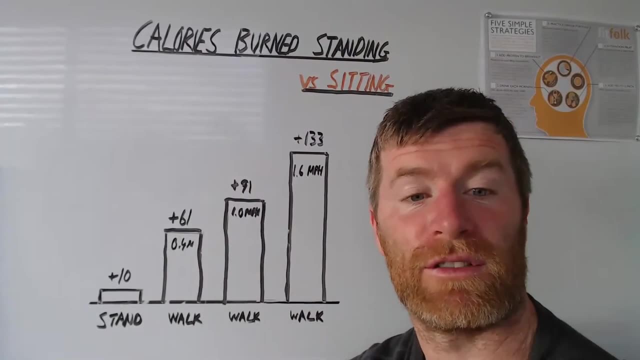 tell as well the rate at which you burn is. you can just tell from your breath. As you start pushing it, you'll burn more calories And obviously then, once you go into cardio, your calorie burn goes through the roof. That's how we. 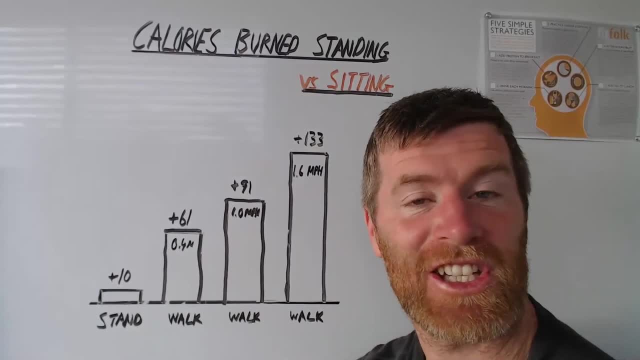 go. Hope you enjoyed that. Check out the cheat sheet and subscribe to the channel. Okay, bye. 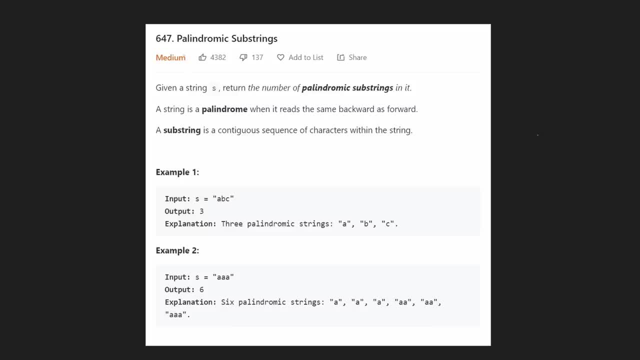 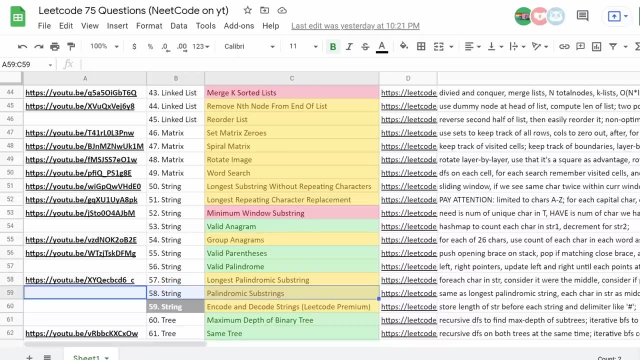 Hey everyone, welcome back and let's write some more neat code today. So today let's solve palindromic substrings, And this is another problem from the leetcode blind 75 list, a list of 75 very good leetcode problems to solve, And this time we will be doing palindromic. 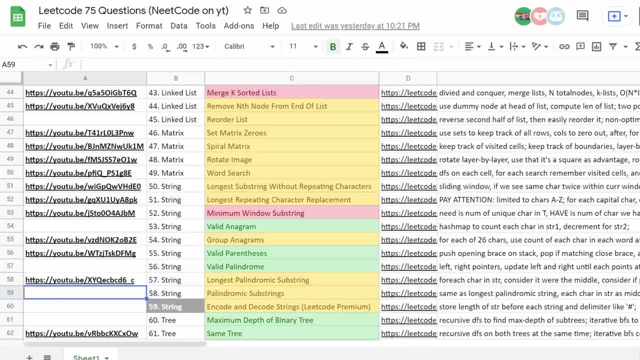 substrings down here, And so we are getting one step closer to filling out this entire list. And this problem- palindromic substrings- is actually really similar to another problem I've solved longest palindromic substring, So if you would like to, I'd recommend watching this. 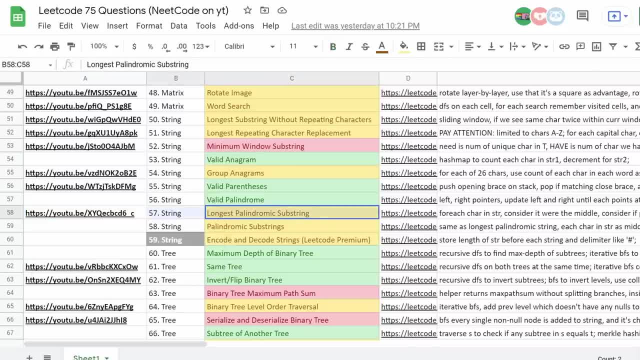 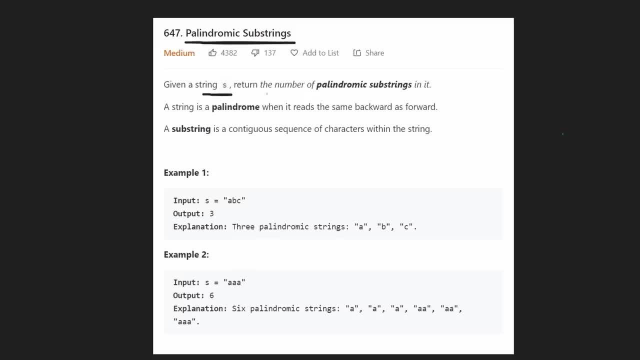 video as well. longest palindromic substring. I will probably link it in the description below. So simply, we are given a string S and we just want to return the total number of palindromic substrings contained in the string S. And, as you may know, a palindromic substring is basically a.